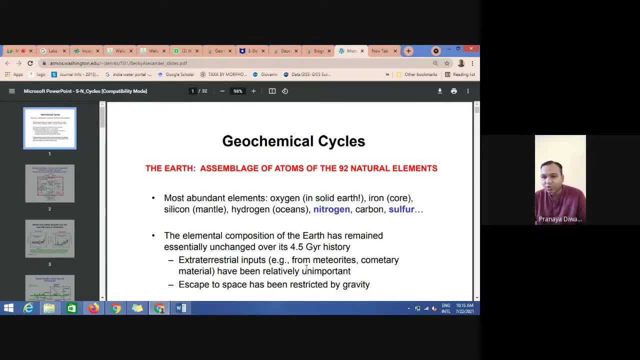 So this is your cycle, a daily cycle, routine cycle. You can also say So again next day you will wake up and all these things you perform at more or less at a different intensity, More or less different intensity. So cyclicity is nothing but a repetivity. Cyclicity is nothing but a repetivity of any process that will be performed by any agency. 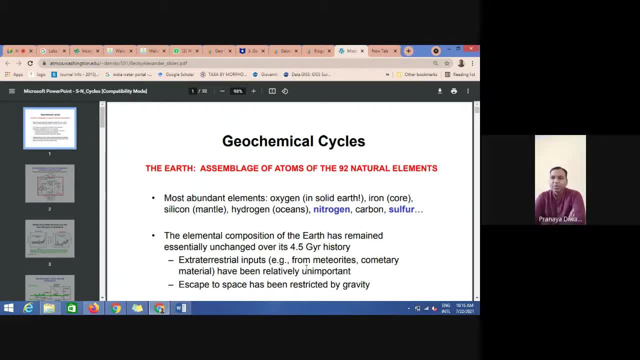 So the earth is an assemblage of atoms of the earth, So the earth is an assemblage of atoms of the earth. The world is a, So the earth is an assemblage of atoms of the earth. 157- 00.. 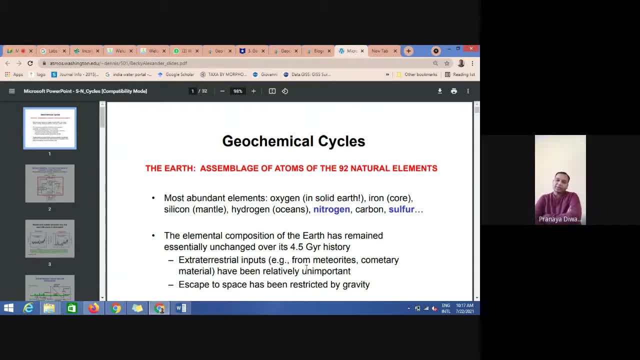 Then there is a cycleelles That cycleelles Actions. Then there is a cycleelles Cylze That cycleelles time. that time maybe it's the 92 elements. presently you have maybe 93 or so. you have to check, update yourself all the time. this question may be ask an. 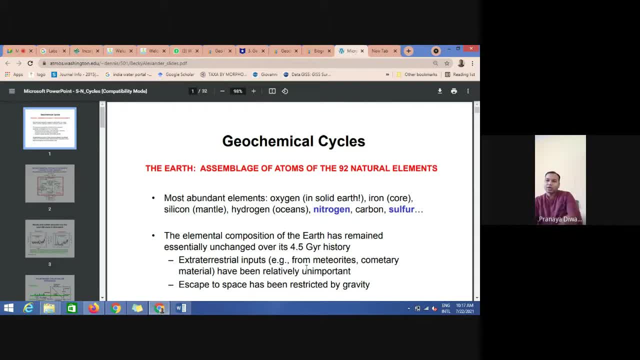 amplitude type question and all. so the earth is having a percentage of 92 natural element. how many elements we have on earth? 92 natural element means all the things which is made up naturally, all the natural things is made up of this 92. in the assemblage of this 92, because you know, that element makes the all your. 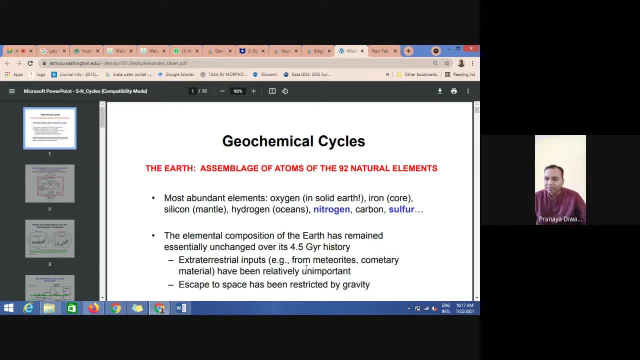 middle middle is a aggregate of the different of your elements, and rock is makeup from the your mineral. this is a part that person is. atom makes the element, element makes the middle middle makes the rock. okay, so this is a cycle, this is a. this is your, what we can say, the of a derivative of one another, then most. 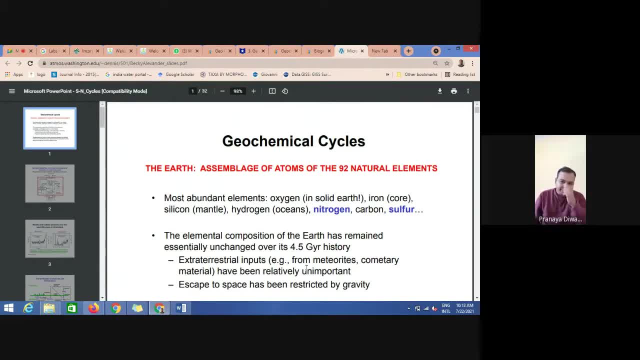 important element and most abundant element is oxygen, whether it is in a surface and whether it is in a subsurface. whether it is a surface, whether it is in subsurface, oxygen is a most abundant element. oxygen is a most abundant element in solid earth. then you have a iron. 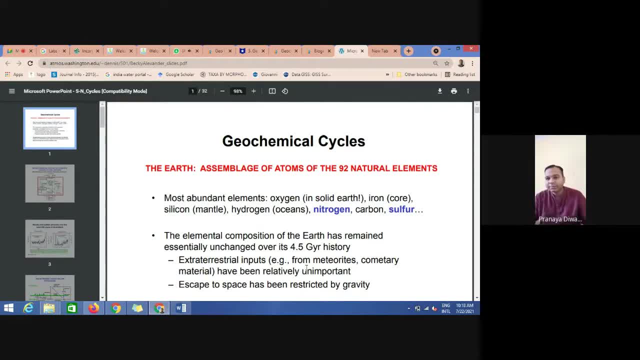 then you have a iron, Silicon, hydrogen, nitrogen, carbon and sulfur. this is a different kind of element. there are difficult kind of element you have that is the most abundant element, what it means, my most abundant element when we are talking about, and most abundant means the percentage-wise, percentage-wise. 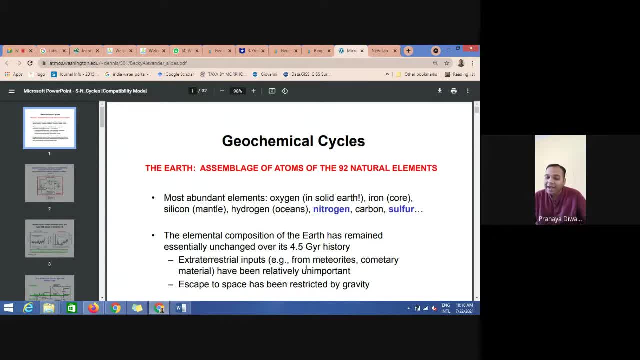 the percentage of this element is highest in the world. so that's why we called us tonic the most abundant element on earth. so which of these elements are most abundant? oxygen, how. the oxygen is more abundant because in atmosphere also you have oxygen. so that is not considered so for this uh criteria. the oxygen is more in a solid earth because you have a most. 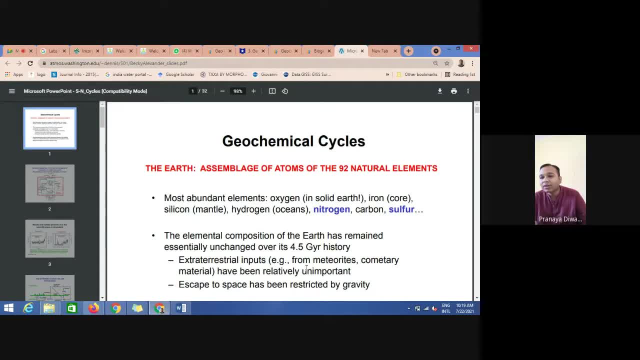 of the rock is formed by the silicon tetrahedra, silicon- mostly. you have a associated with the oxygen that is called as a s i o 2 tetrahedra- s i o 2 silicon oxide. silicon oxide is a term which is used for this one. so silicon tetrahedra is a term which is used for this one. 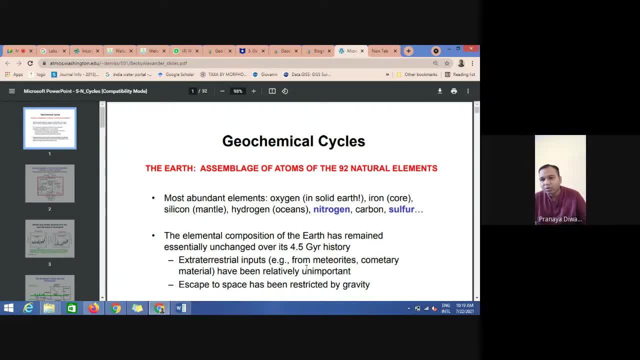 then you have most abundant element. then you have most abundant element: uh, oxygen, iron ore, silicon, oxygen, iron ore and silicon. so uh, oxygen is mostly abundant in your crust because you have a silicon oxide mostly abundant in a crust. then you have iron in core and you have iron in fourth: silicon in metal, silicon, metal, hydrogen in the ocean, nitrogen. 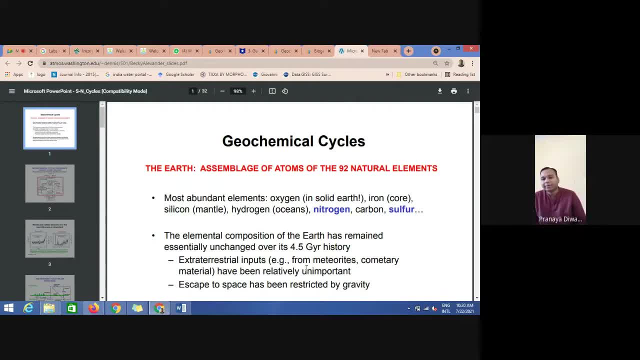 carbon and sulfur. this is a different kind of element. you have the elemental composition of the earth. the elemental composition of the earth has remained essentially unchanged over its 4.5 billion year history. the elemental composition of the earth has remained essentially unchanged over its 4.5 billion year history. extraterrestrial input: extraterrestrial input from meteorite. 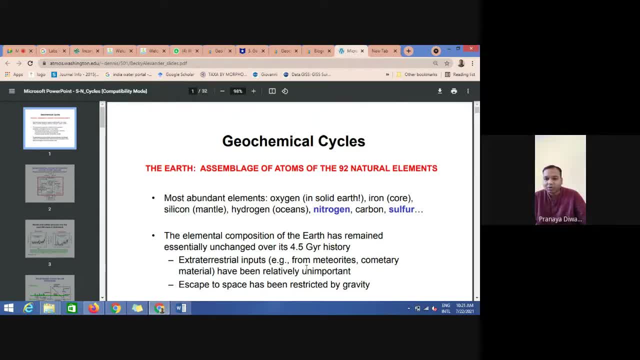 cometary material have been relatively unimportant, so the elemental composition of earth has remained essentially unchanged. so you know, we already studied in a previous lecture about the what uh thermodynamics law. so you, you can have, uh the, you can have the thermodynamics law and the. 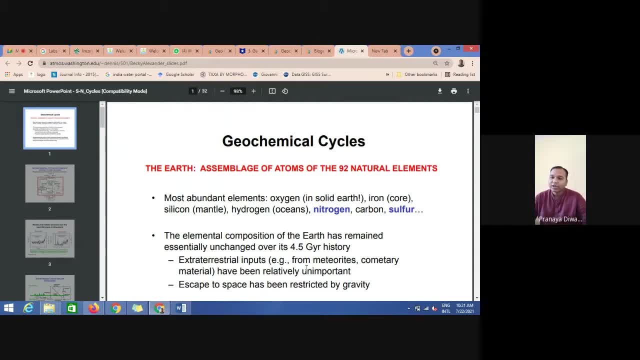 what the thermodynamics law suggested. the thermodynamic law suggested the, the energy, and this one is neither be created nor be. not the energy neither be created nor be destroyed, just change from the one is a part to another part, and that's why there is coming a change in just language and language definition. 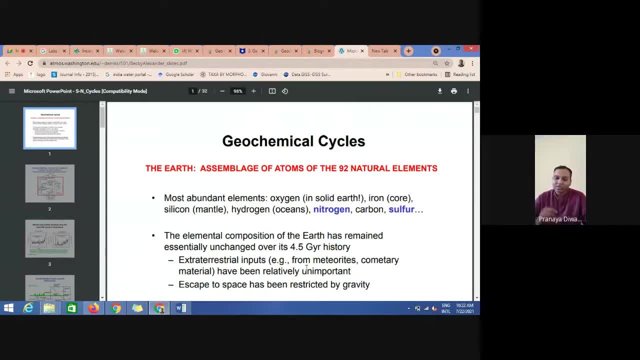 here only because you only have one after an other, the natural phenomena back to you. theêu finance also recorded that energy neither be created nor be destroyed, just change from one part to the another part. so this is your geochemical cycles. uh, so this is the your. what we can say? the 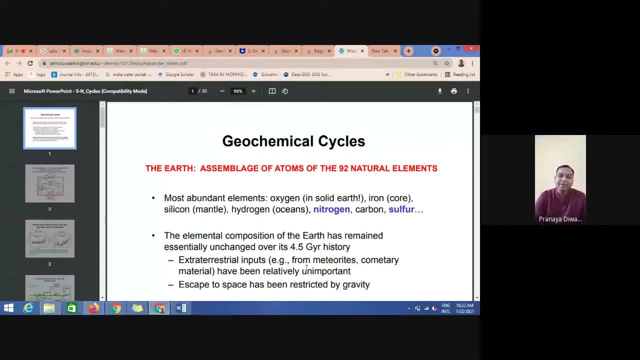 this is uh what we can say. uh, this is uh also. uh, this is also uh, this is also you can say for the elemental element, neither be destroyed nor be is just convert from one part to another part. that's why it is called as the cycle. that's why 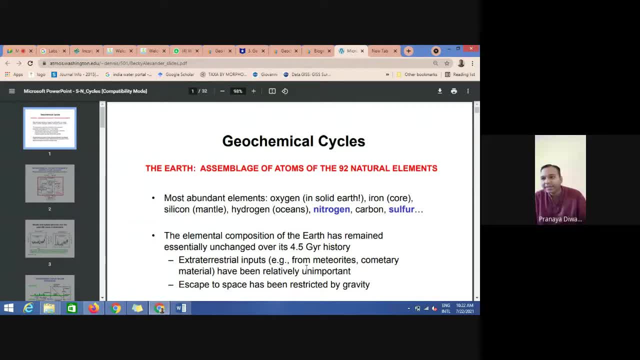 it is called as a cycle. so geochemical cycles are those. geochemical cycles are those, like you have a what we can say the water cycle. okay, like you have a hydrological cycle or water cycle you can see. so what is the hydrological cycle or water cycle can tell you about? or what, how it is started? 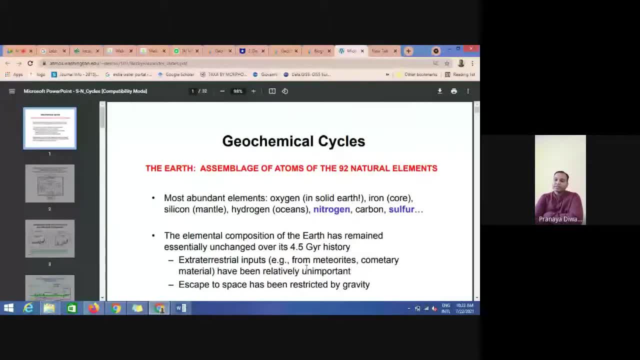 and ended. a water cycle is like: you have a water in form of lakes, ocean and all. then it gets evaporated by the, your heating, then it is get to the cloud, cloud again, get condensed and get this one into the surface. this is what you can say, the, this is what the assemblage, this is a, what you are, a. 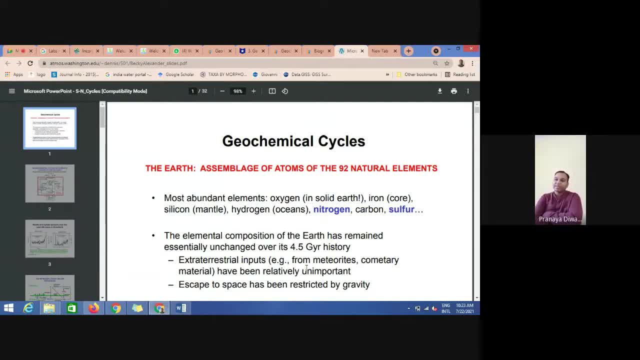 cyclicity is there how your side it is, there is repeated action. so as for as the element of the earth, that ninety-two element in the earth, its constant from the last four point five billion years history of that, you know, that render, or this form, okay, whereas the extra. 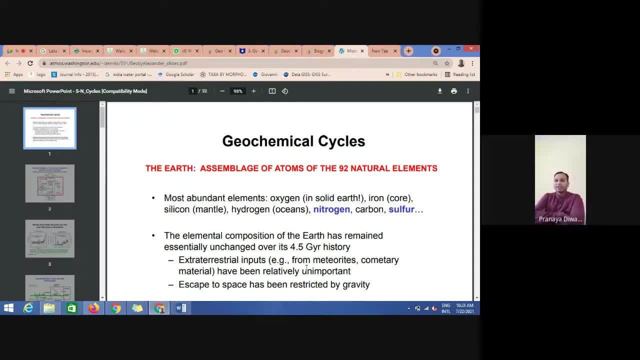 traditional. you know that some maturity impact is also there. some maturity impact will not fall that much because most of the most of the element or most of the, this one is already in most of the element already been not catched by or it get destroyed in the outer space. okay, 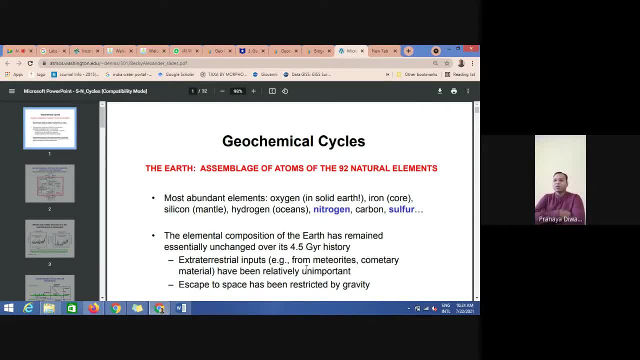 destroying the outer space. you know that when you study the atmosphere, what is the ozone layer? and all this one does work of this one to destroy the metronomy right in outer space only if that is not there, if the that outer space is not done this work, you get a metric impact daily. you can see that the 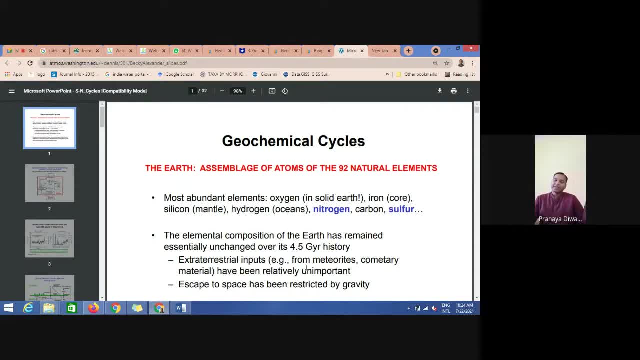 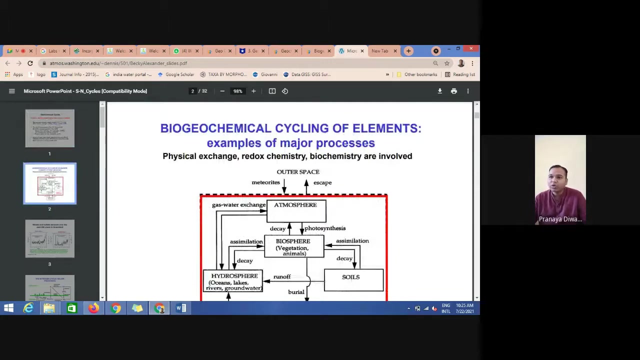 space is open. the space is open. if this layer is not there, they make right is daily get travel. you know a lakhs of a thousands of better rights is get travel, but they are not supposed to fall on the earth because of this outer material, out of action. then we have biogeochemical cycling of the 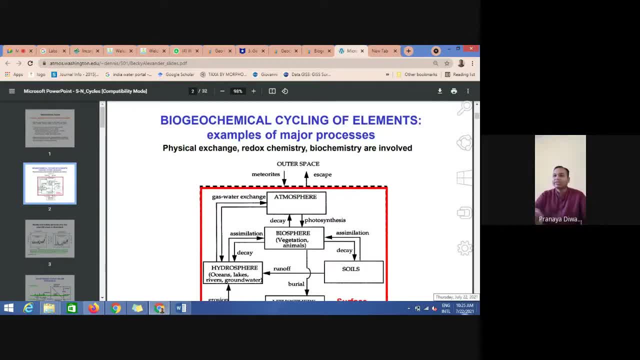 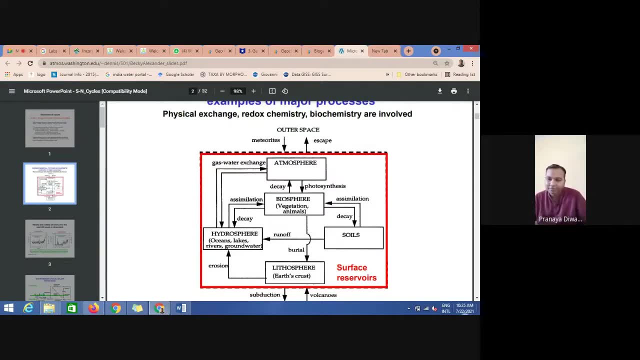 element. example: the major processes. so this is how the process is get, how this process is get, how this어요, how this is. so this from the didney to get the spread from the earth right. this way he can do it from the earth. in biosphere you have a hydrosphere, lithosphere and soil. okay, atmosphere, biosphere, hydrosphere. 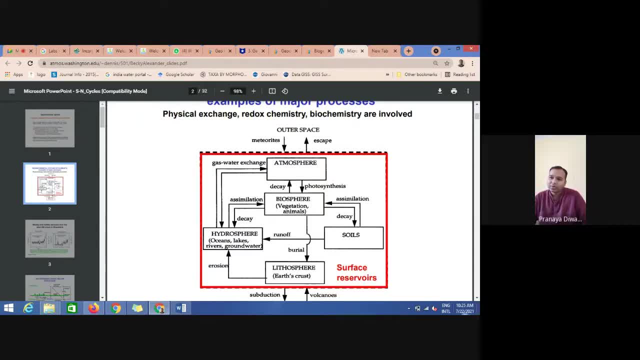 lithosphere and soil. so, uh, what is the lithosphere will be do? when you have a lithosphere, you can have the? uh erosion activity, you can have the erosion active, erosion activity and erosion activity will be take. uh, erosion activity will take the element into the ocean, lakes, river and 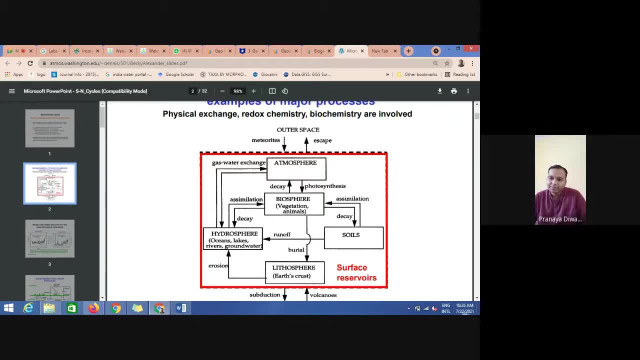 groundwater. you know that, uh, the erosion activity, and all this one, is very much important for the formation of rock. so look, when the rock is formed, you have a erosion activity. what that erosion activity will do? it will uh take your element and minerals into the hydrosphere. 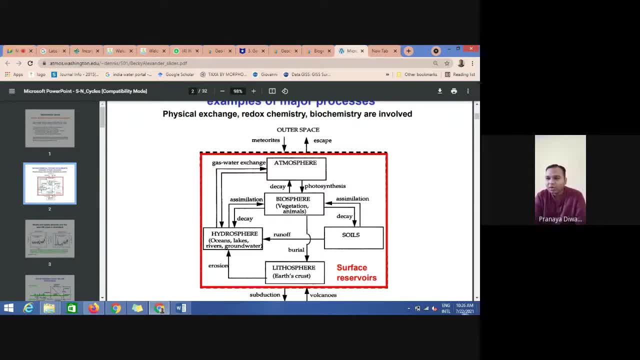 into the hydrosphere. so, uh, hydrosphere is nothing but a water bodies, whether it is the ocean, whether it is the ocean, whether it is the lakes, river and groundwater. so this is a different kind of this is a different kind of uh, uh elements we have. this is different kind of element we have. so, uh, then this one is get. 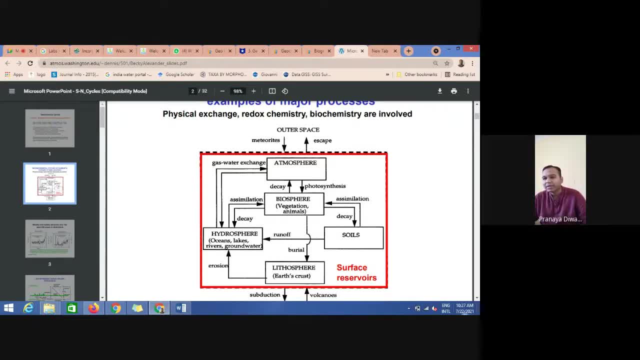 uh, this hydrosphere from the hydrosphere. you know that water is also get to the uh other sphere by the water cycle. so hydrosphere will go to the biosphere, hydrosphere will be go to the biosphere. then in biosphere, what is the? what is the? 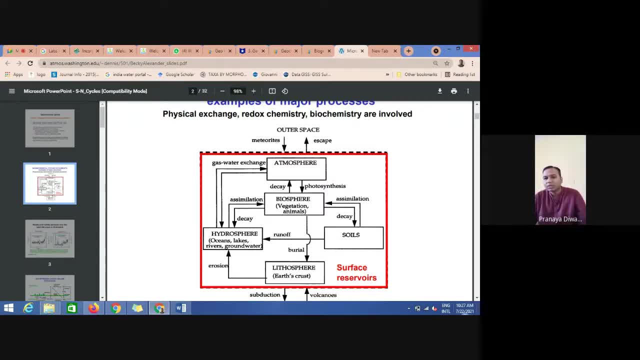 the component of biosphere. you have vegetation, animal and all you have vegetation animal and all that is known as your biosphere. then you have atmosphere, then you have uh, then from the biosphere it goes to the atmosphere. okay, then from biosphere it goes to the atmosphere, if from atmosphere it. 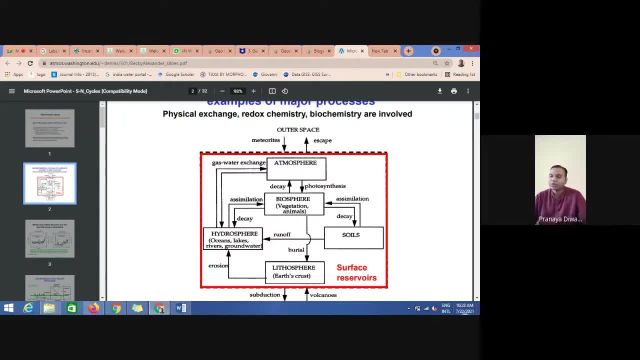 again go to the, your hydrosphere. so then from atmosphere it also goes to the uh biosphere. after yeah, aquellas, it will, goes to the soil, then Wirtschaft. so this is a cycle. elements can only go from, or went from, the one side, one part of the or one sphere to 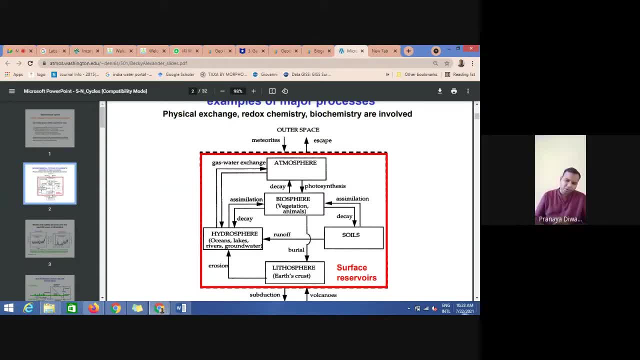 the another square. it cannot destroy, it cannot get, create it it cannot, because, whatever the things are created, you cannot call them a mineral. mineral is the definition of this homogeneous substance. the first word is very important. naturally, offering cannot make in a machines and in a market, or you know, your this one. 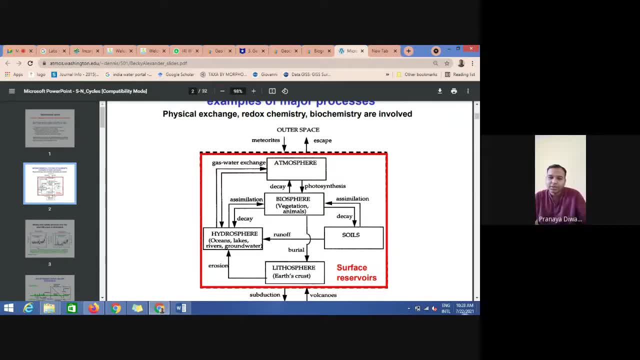 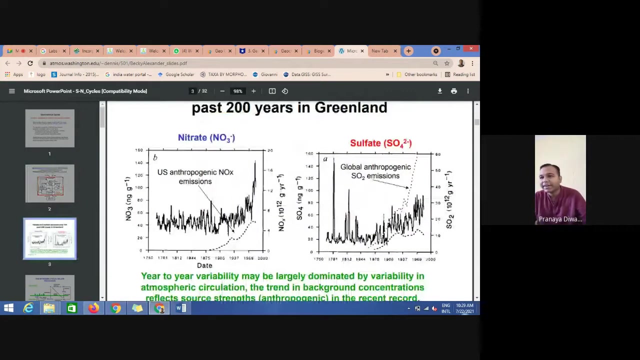 so. So this one is known as the at Lithos cycles, and so you can have the Mineral in form of window. you can have a cycle for this one. So physical exchange, redox, chemistry, biochemistry is involved in this. all the This Is how the nitrate and sulfate aerosols over the past 400 years in a green land. 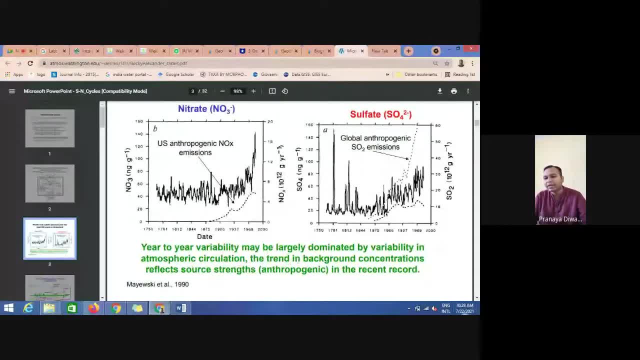 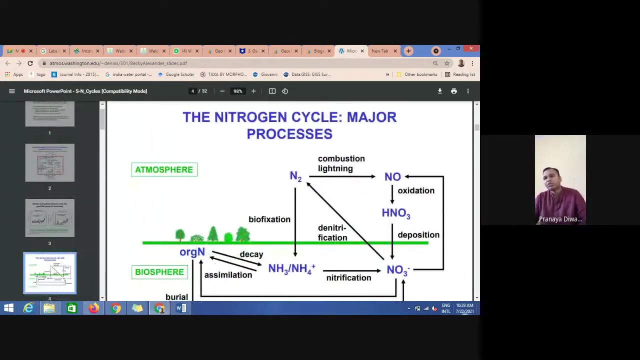 Here. And the training background concentration replaced the source strength in the Resilient record. so here we are, a beauty largely dominated by a very clean atmosphere. some pleasure. the trend, the trend in background concentration reflect the source strength in the recent report, The nitrogen cycle, What so? now you have a different element. 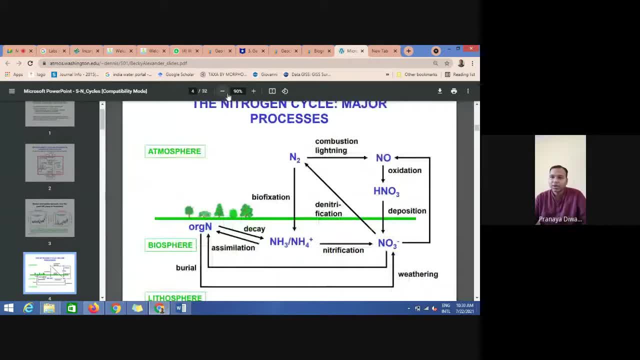 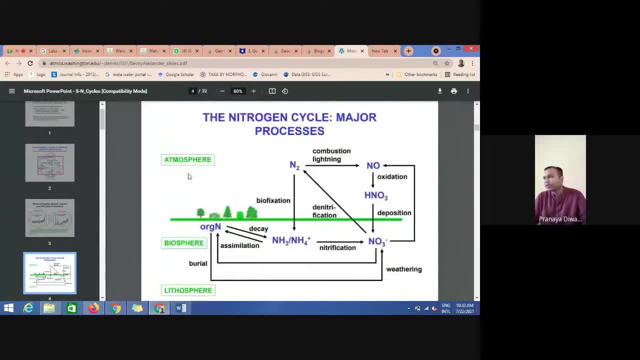 You have oxygen. You have oxygen. You have a nitrogen, you have a nitrogen, then you have a Hydrogen. all this one, You have a carbon. all this one have a Cyclicity, all this one have a cyclicity. so atmosphere, from the atmosphere, it is get to the 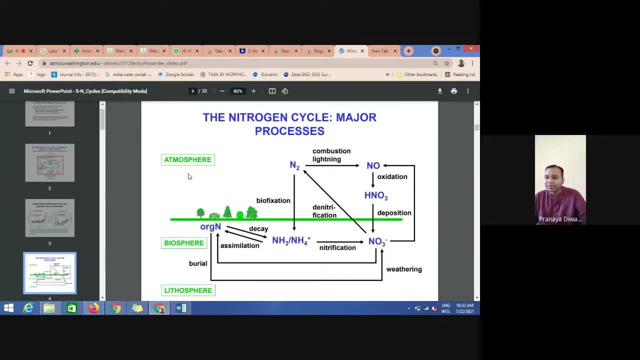 So you can start from the weathering process again. so when there is a weathering process you have a nitrification process. From the nitrification you can directly convert to the N2, or by the some of the different American Oh. So At crazentis. 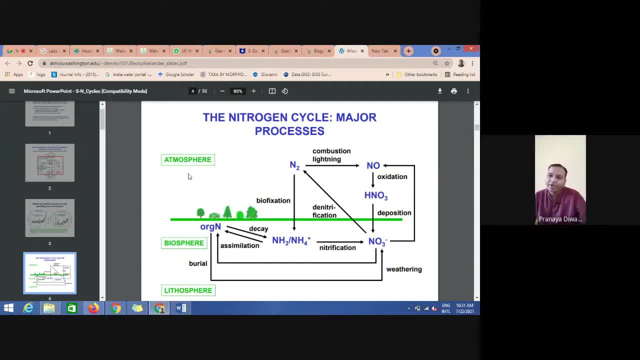 At work, So this went in you. things like nitrogen also. people is attached organically on nitrogen as well, as the oxygen in nitrogen is always attached. the nitrogen is always attached to the another nitrogen nitrogen and another mineral is attached to the another elementy. This is An diferent 언 Stevie beef. 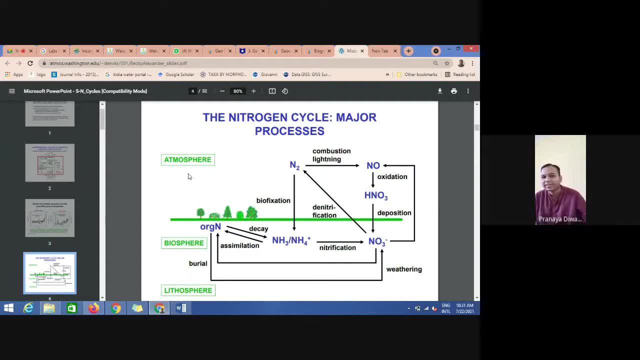 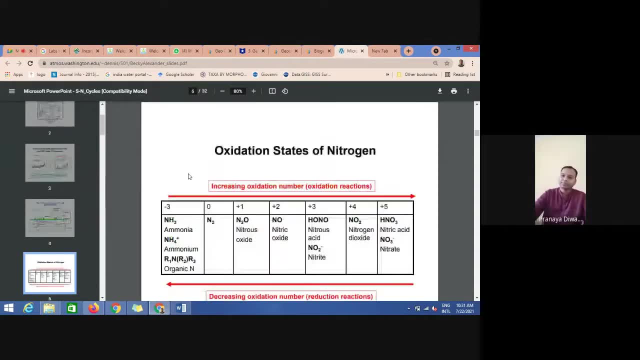 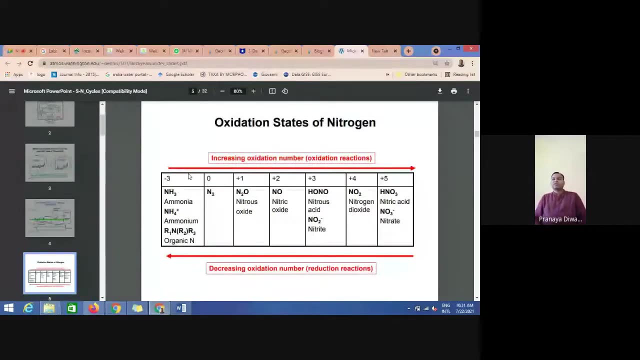 In case of oxygen, you have a silicon oxide, SiO3 or SiO2.. So that is what you can have. Then you have oxidation state, Then you have oxidation state of the nitrogen, So you have NH3.. You have NH3, that is ammonia. 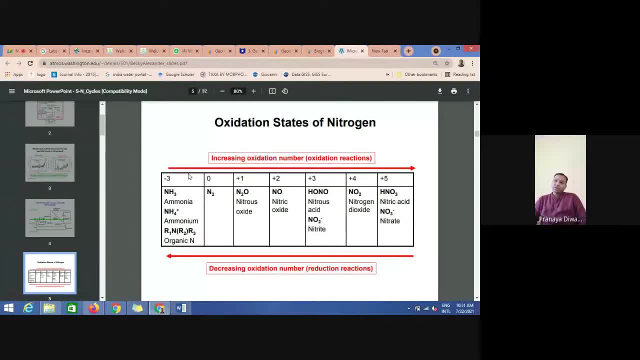 Then NH4, ammonium. So this is an increasing oxidation number with a decreasing oxidation number. So oxidation state: when you combine the nitrogen with the oxygen, you have a different element. You have a different element, Like on the carbon also you can have a carbon, as you are seeing. 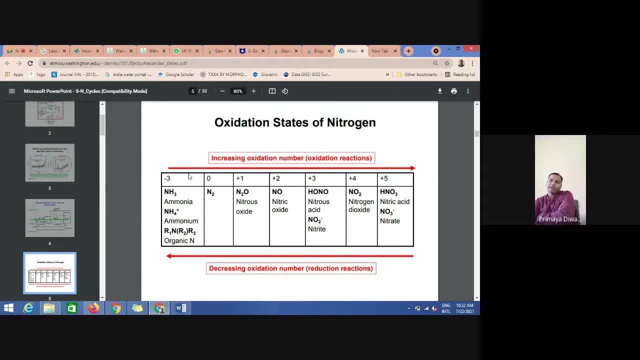 Then you have a CO2.. Carbon monoxide, CO2, carbon dioxide. This is how you can have a different element, Different element in your cycle. So if there is a zero nitrogen oxygen, you can have. it is known as a nitric. 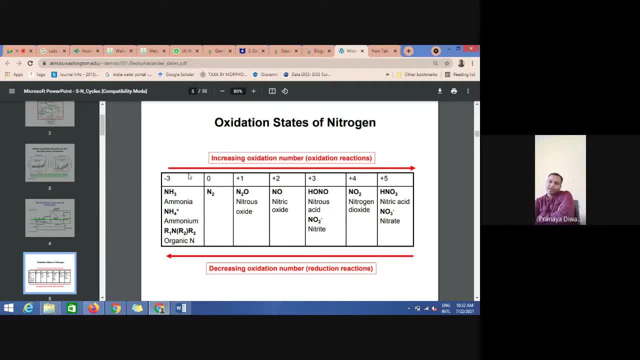 It is known as a nitrous oxide. That is called as N2O. If there is a two oxygen, Okay, if there is a two oxygen, then you have. it is called as a nitric oxide. It is called as a nitric oxide. 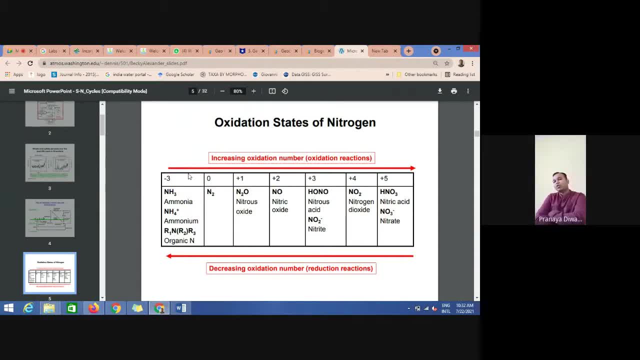 Then you have a nitrous acid, HONO. That is very well known as nitrous acid, That HO2, NO2, that is a nitrate, NIO2., NIO2., NIO2.. So that is known as your. 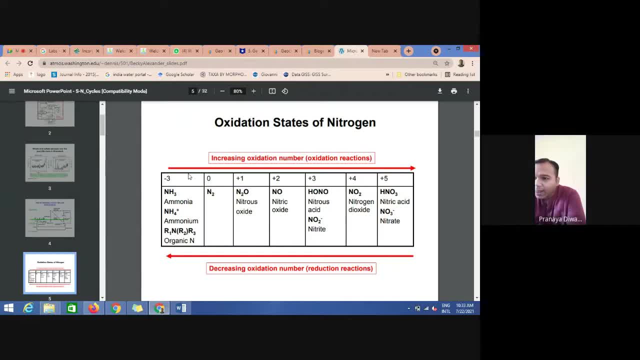 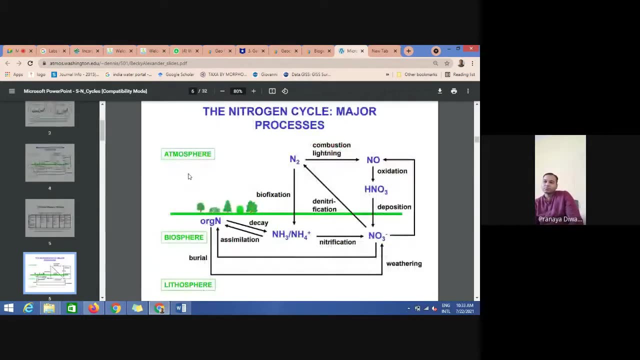 NIO2, sorry, NO2, that is your nitrite. NO2, that is a plus four. You have a nitrogen dioxide. So this is a different state of oxygen in the nitrogen And this is how your nitrogen cycle will perform. 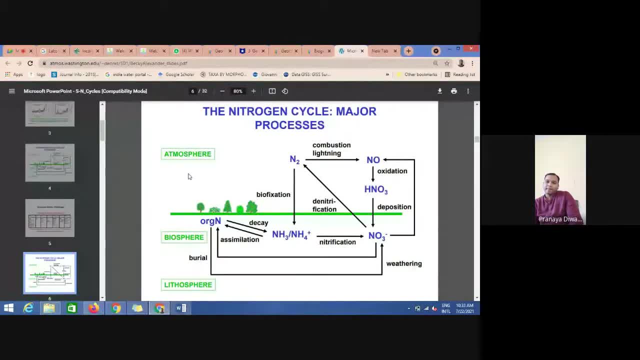 How the nitrogen cycle will look like. So how the nitrogen cycle will be. So you know that atmosphere is contained as more than 70% of the nitrogen, So the atmospheric nitrogen is also very important. So you have. So all about and, at the last, what I can say you. 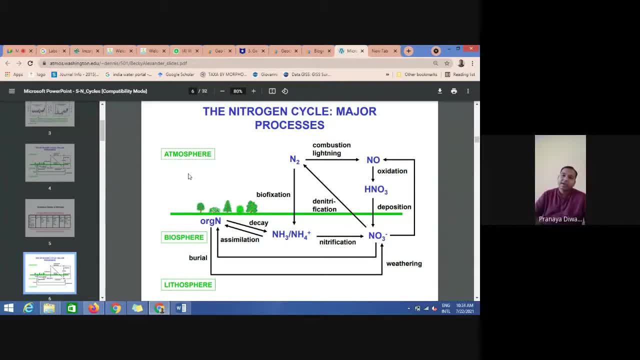 Cycle. cyclicity is a repetition of action Plus. in cyclicity you can say that The element is from Recycle from one class to another. One class means one sphere: From atmosphere to biosphere, from biosphere to lithosphere. 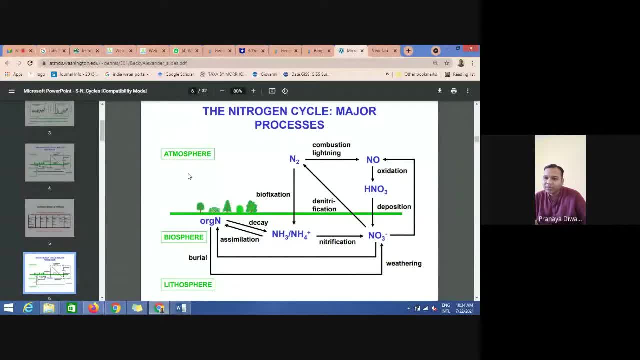 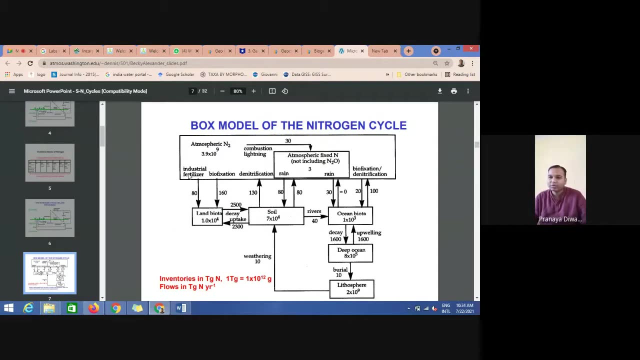 So this is a difference here you can have From this difference here you can, You can have this cycling process. This is a box model for the Your nitrogen cycle. This is a box model for the. This is a box model for your nitrogen cycle. 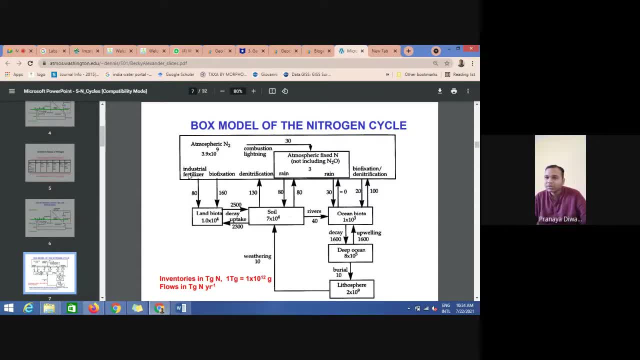 This is an atmospheric ENCODE. This is an atmospheric ENCODE. Then you have combustion lighting. You have a combustion lighting, Then you have atmospheric FIXED D. So this is how you can have a nitrogen cycle. So this is the box model before we can see the nitrogen cycle: major processes. 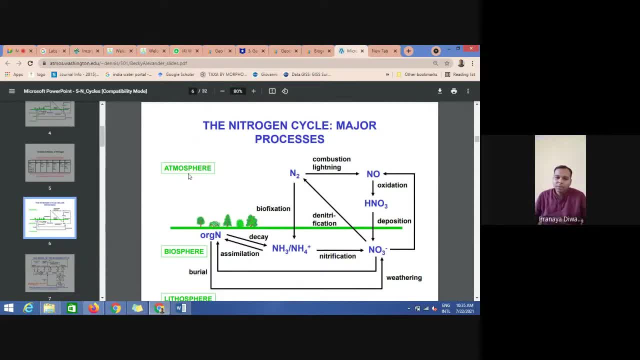 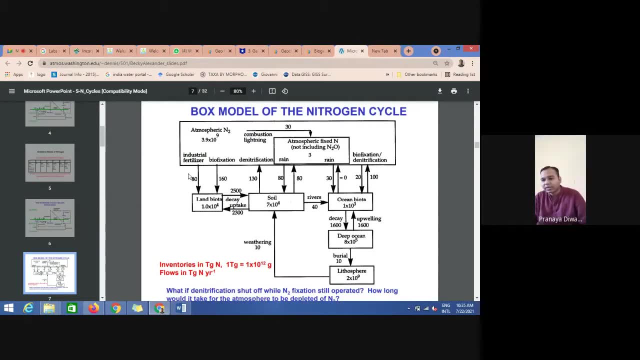 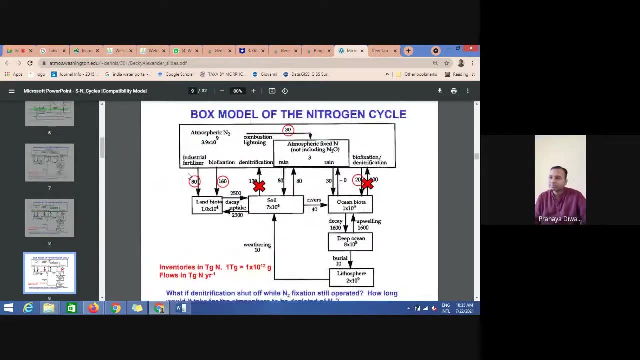 What is the major processes behind the cyclicity of the nitrogen? Then you have a box model of the nitrogen cycle. Then you have a box model of the nitrogen cycle. Then you have an atmospheric ENCODE. Then you have an atmospheric ENCODE. 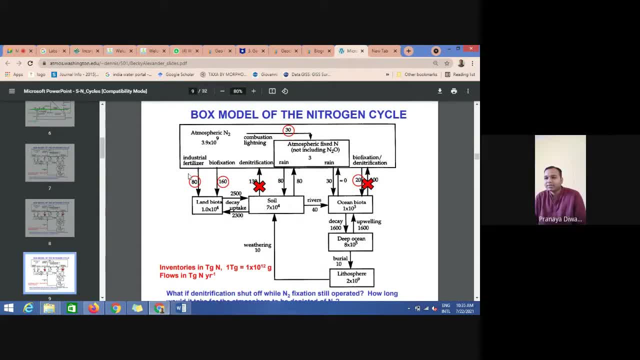 Combustion lighting, Combustion lightning. Then you have a bioplexation, So different kind of process which is involved in a nitrogen cycle. This is the emission of the nitrogen in a electrosphere. So you can see the number of percentage of the element of nitrogen in a heterogeneous. 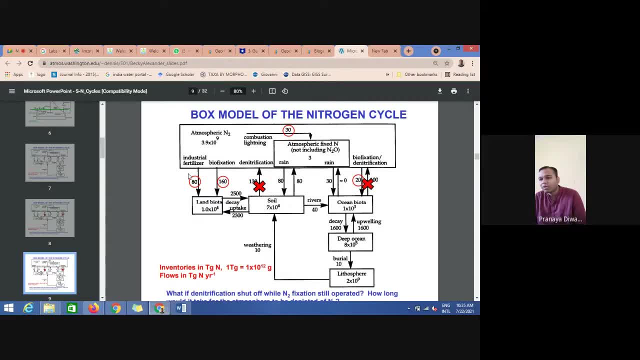 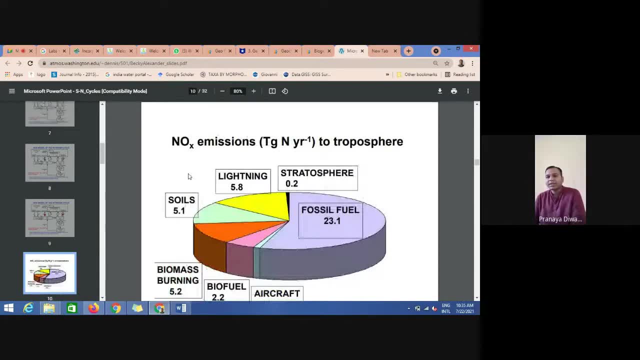 cycle. So you can see the percentage of the element of nitrogen in a heterogeneous cycle element. so five, one percent is a because of the sign possible. so the is like this status beer possible and this one. so in the possible also you have a 23%. 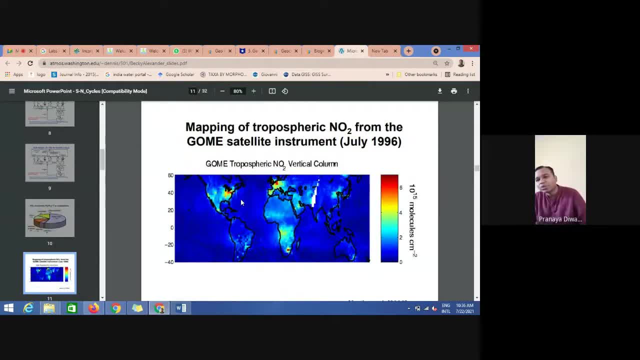 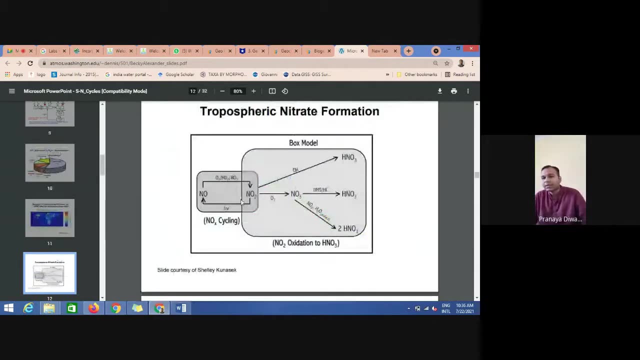 with the remote sensing and GIS also you can map the proposed very nitrogen oxide from the earth different satellite. so this is what you are mapping of the proposed very natural formation. then you have a nitrate formation. so this is a picture which is suggested, that earth tropospheric nitrate formation, how the tropospheric nitrate has been formed. so 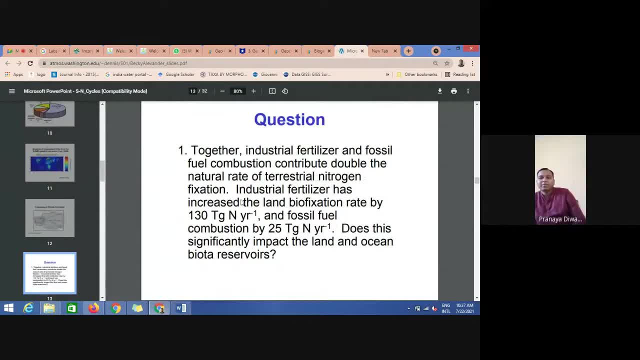 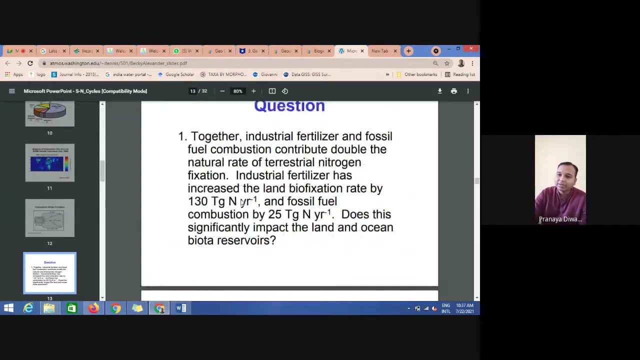 what is the question? the question is: together the industrial fertilizer and fossil fuel from combustion contribute double the natural rate of the fertilizer- had increased the land bio excision, although, although the- what we can say- the data is significantly impact the land, and this is a a box model. what the nitrogen? 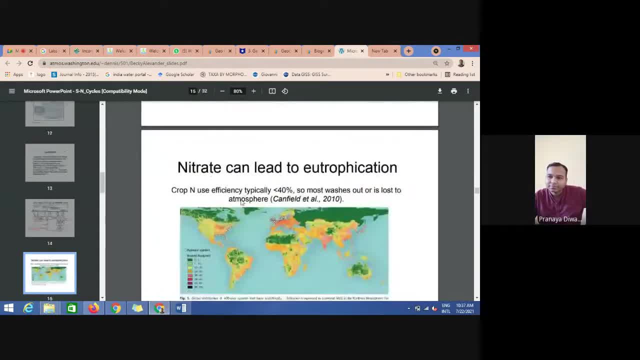 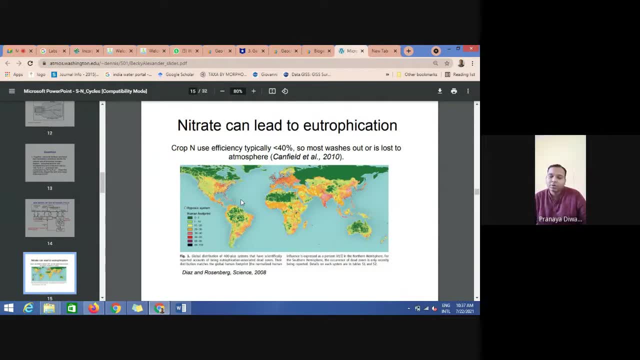 Again a box model for the nitrogen cycle. nitrates can lead to eutrophication. now you can need to know a simple word. what is mean by eutrophic release, eutrophic release, eutrophic release, what we say? so eutrophic release is the eutrophicton gas, so it is from eutrophic value to the energy. 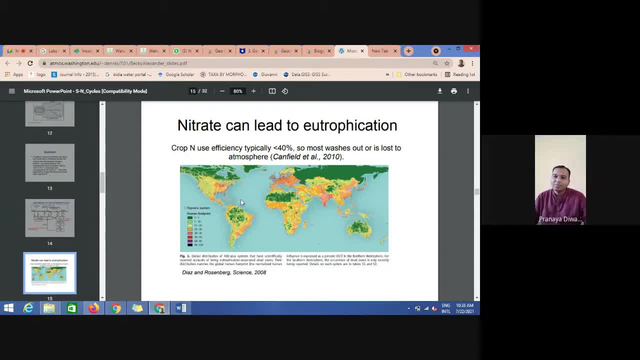 eutrophication. eutrophic, mesotrophic and oligotrophic. This is the three different type of condition of any water body where you have algae, and all Eutrophic, mesotrophic and oligotrophic. Eutrophic, mesotrophic and oligotrophic. 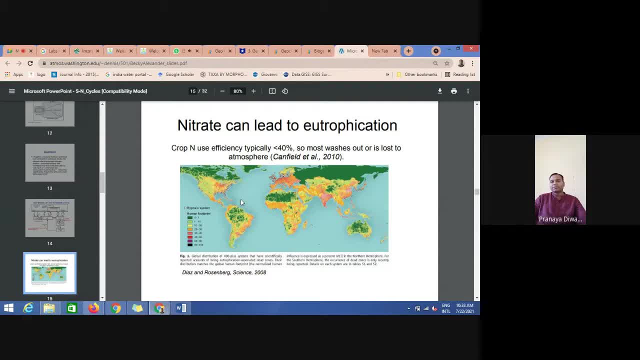 So eutrophic is nothing. but when you don't have crystal clear water, When you don't have crystal clear water, that time you can say that this water is contaminated. Coffee and glass So. so nitrate can lead the eutrophication. 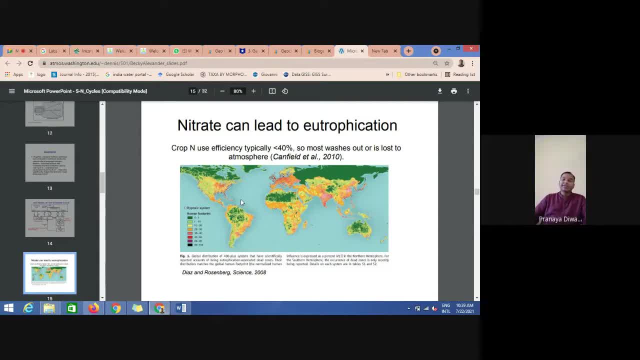 It is said here, nitrate can lead the eutrophication. Why it is need to increase the eutrophication? Because nitrogen is also part, or is also a food material for most of the creature. Okay, So eutrophication is increased when there is a algal growth, and this one. 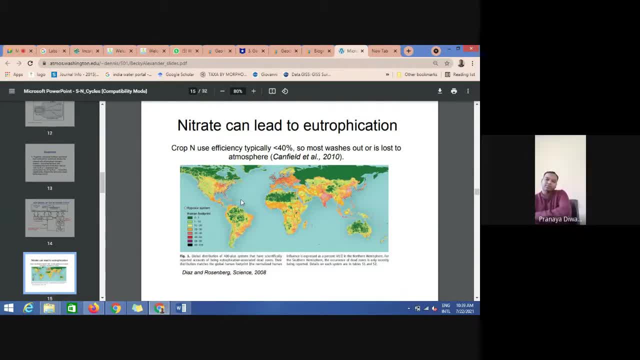 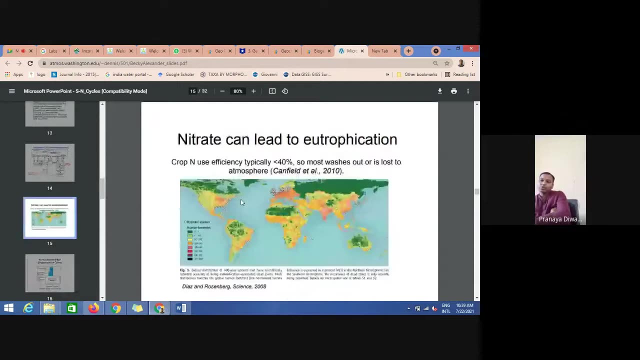 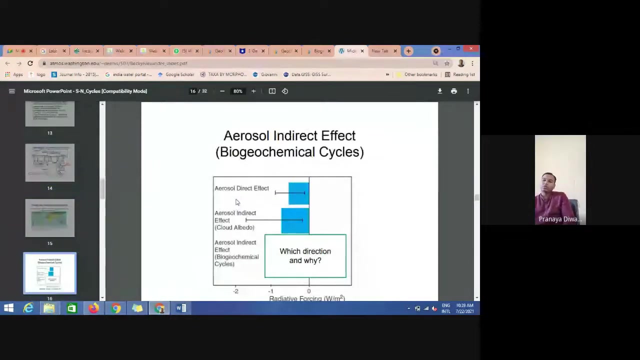 You have a different parameter like such depth and all. You have a different parameter which measure this eutrophication. Then you have aerosols. Then you have aerosols, indirect effect, biogeomical cycle. Then you have indirect effect on biogeomical cycle. 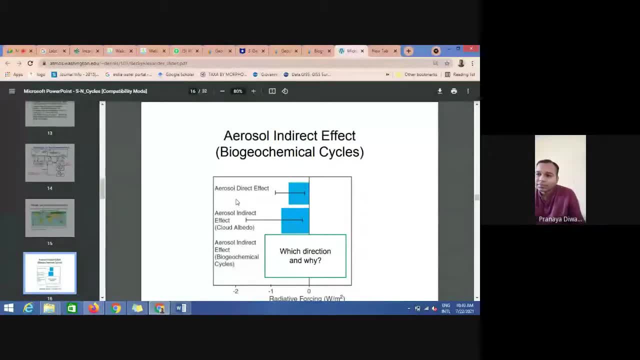 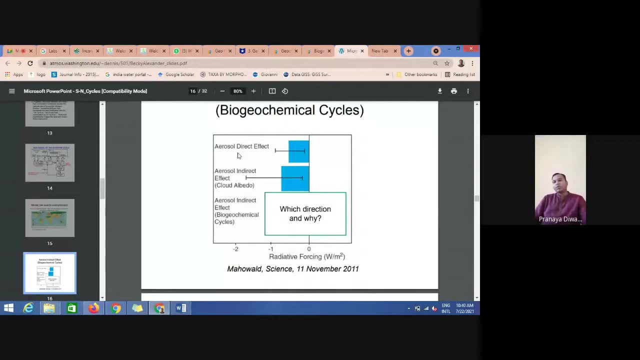 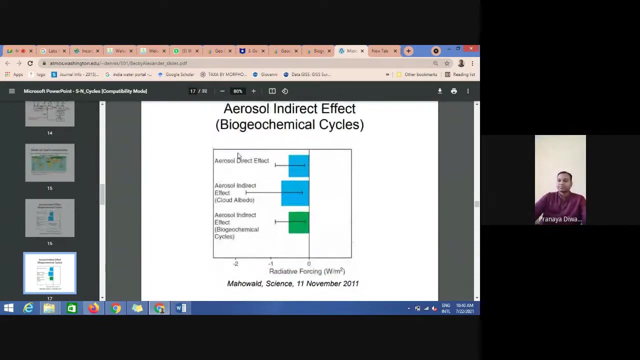 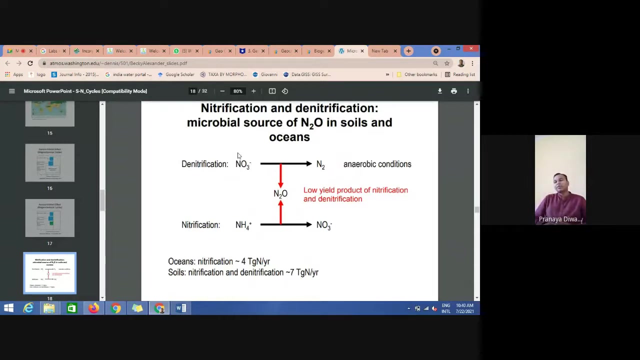 So we call this as lateral sound. So we have aerosol. What is aerosol? What is aerosol? Aerosol is an aluminium alloy. What is aerosol? What is aerosol? What is aerosol? so the nitrification and denitrification microbial source of N2 in a solid, and so you have denitrification. 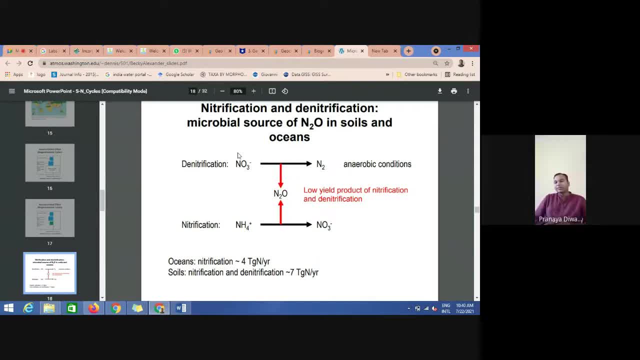 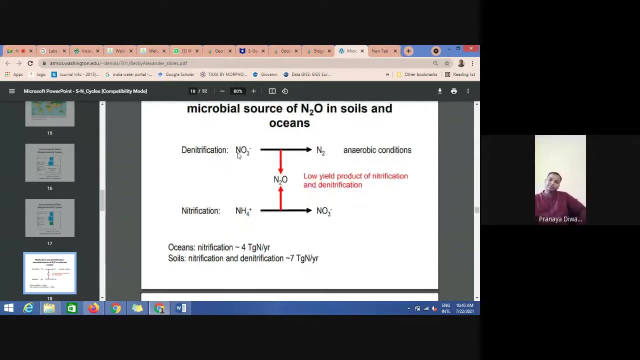 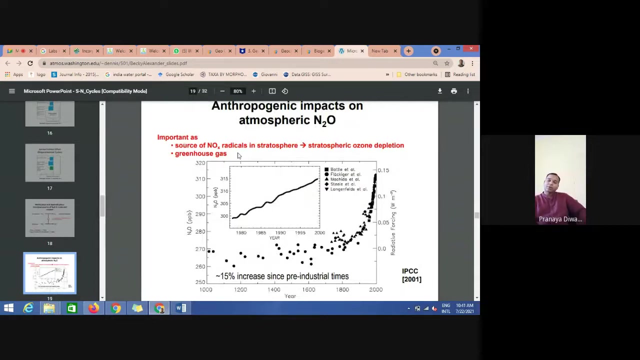 denitrification, anaerobic condition, so you have denitrification, nitrification, so it will be formed. it will be formed as well as destroyed this element. so what is the impact of atmospheric and what is the impact of? what is the impact of anthropogenic impact of? 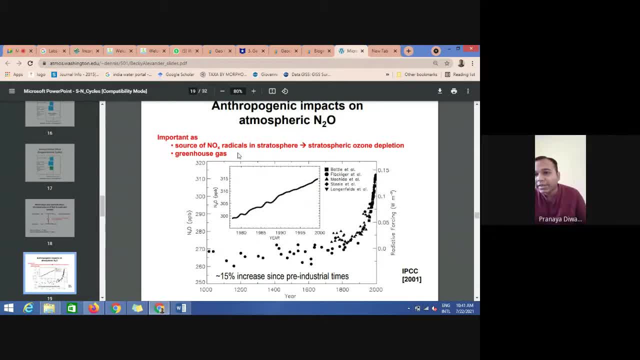 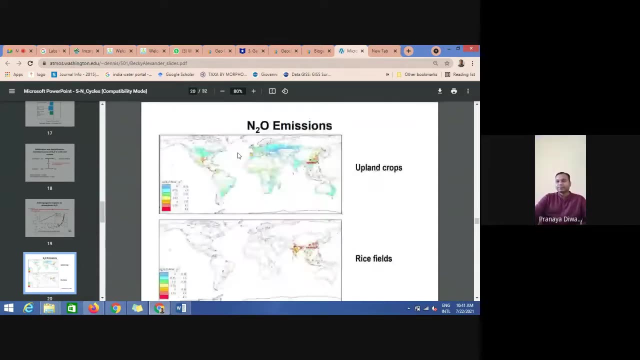 so source of nitrogen radicles in a stratosphere, stratosphere ozone depleted in green south gases. so nitrogen is as coming from the nitrogen is considered as coming from the base. do you have a nitrogen emission? this is the upland crop and this is the rice fields. 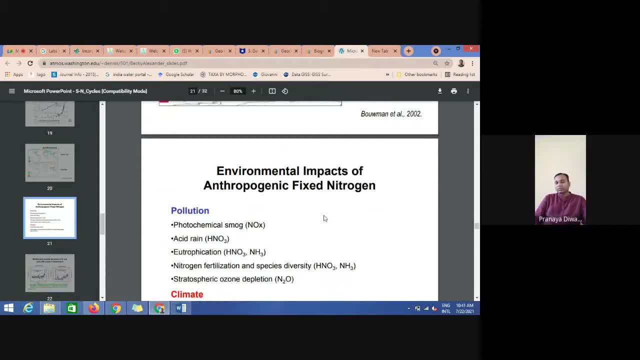 then what is the environmental impact of anthropogenic fixed nitrogen? there is a major impact. your photochemical smoke, acid rain, okay, acid drain is nothing, but when you have more excess acid is there. so so your environment is mostly impacted by this anthropogenic fixation for the nitrogen. 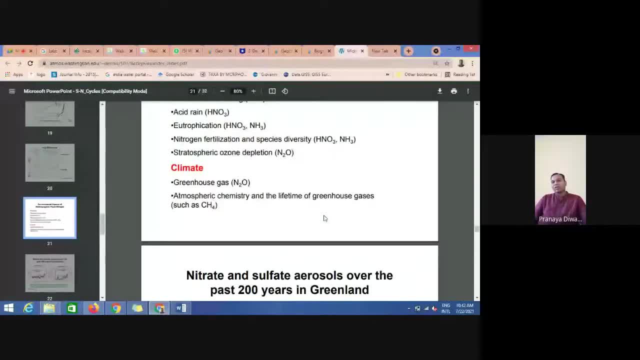 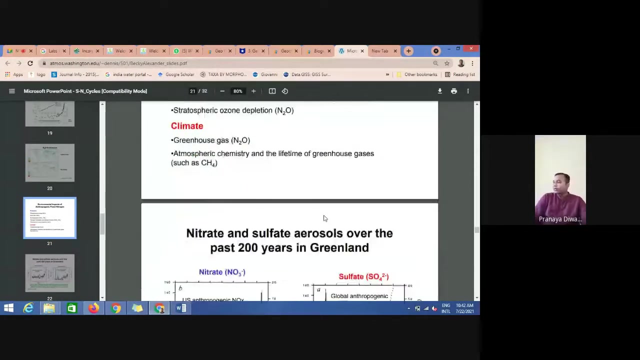 then climate? what is the climate climate? you know that a long term average weather condition is known as climate. long term average condition is known as climate. Then you have greenhouse gases, then you have greenhouse gases. so what is greenhouse gases? So greenhouse gases are the gases which are very important for this one. 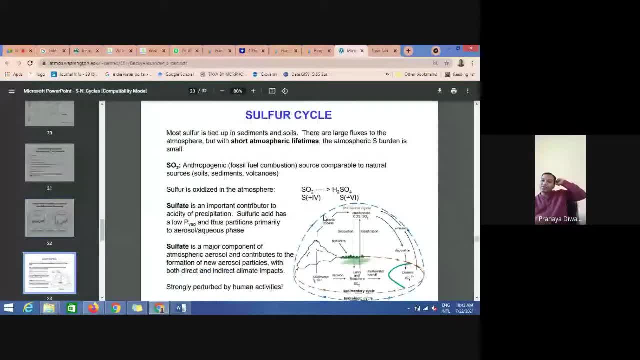 Then next you have sulfur cycle also. So likewise, likewise the nitrogen cycle, you have a sulfur cycle also. Most sulfur is tied up in a sediment and soil. Most sulfur is tied up in a sediment and soil. There are large processes to the atmosphere. 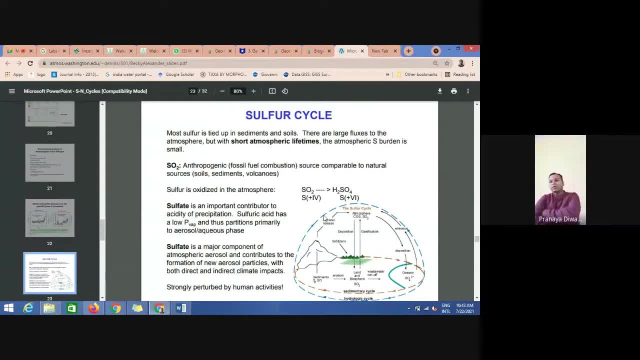 There are large Success to the atmosphere. but with short atmosphere lifetime The atmosphere S is Okay, So most sulfur tied up the sediment and soil. There are large fixes to the. There are large fixes. There are large fixes to the sediment and soil. 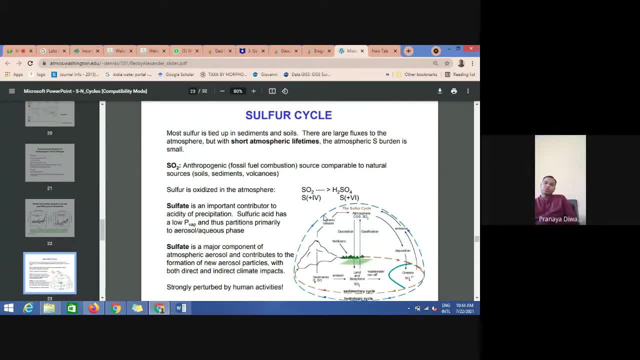 Those two are the most difficult to get. The most difficult one is sulfur dioxide- SO2- sulfur dioxide- Anthropogenic source comparable to the natural source. Anthropogenic source compared to the natural source. Sulphur is organized in the atmosphere. Sulphur is organized in the atmosphere. 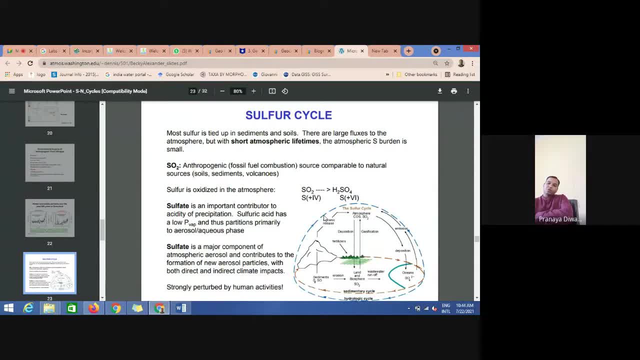 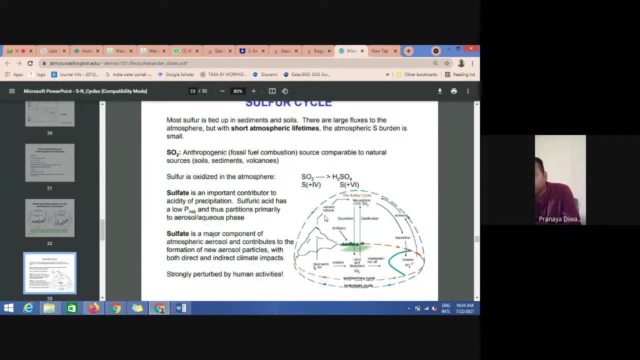 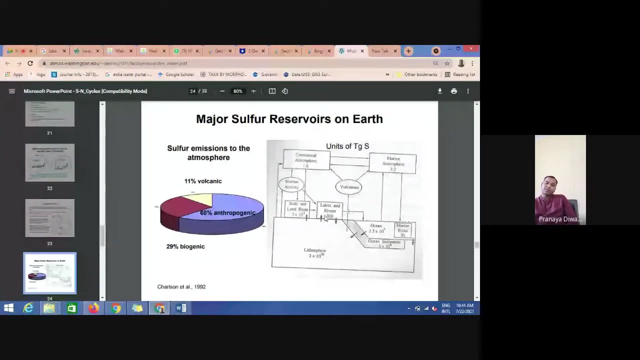 Then we have surface. It is an. This is a sulfate. then you have a sulfate. okay, sulfate is the important component of atmosphere aerosols. so here you can see the most major sulfur which I can: 60 percent of the atmosphere, nitrogen is. you can see the remain. enough ocean, sorry, yeah. 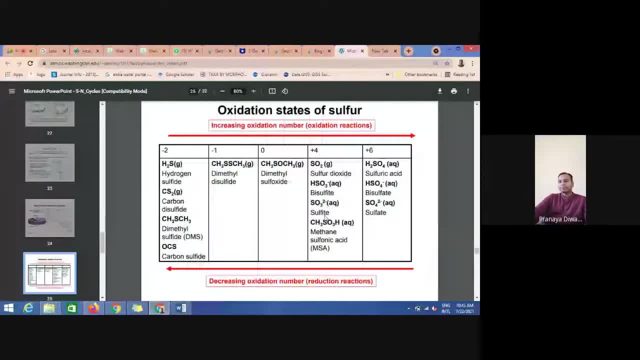 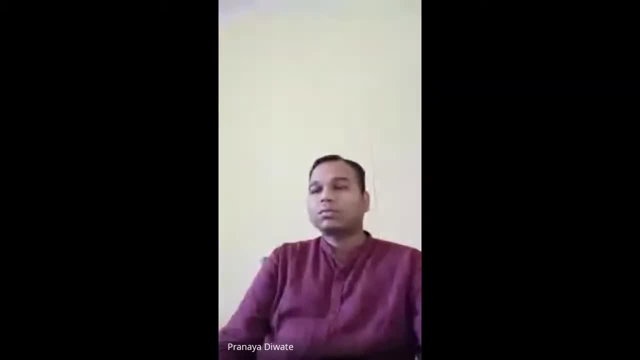 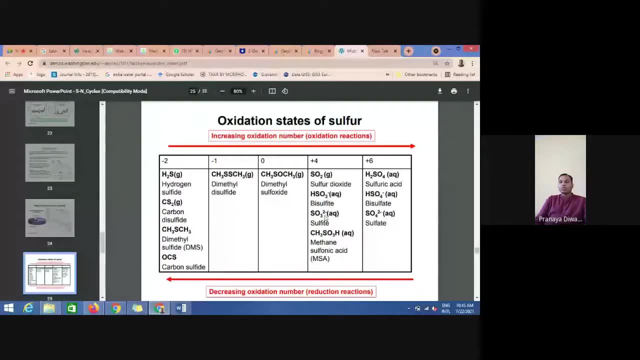 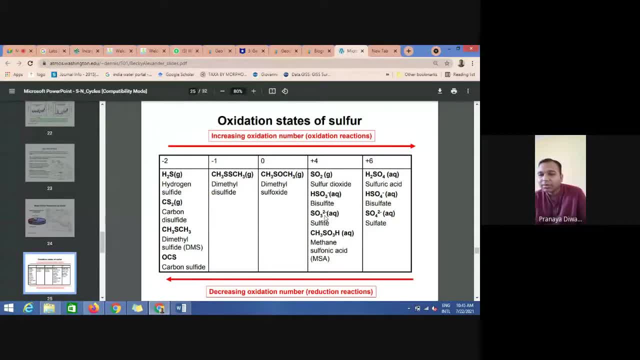 sulfide carbon, di-di-sulfide d-methyl- d-methyl, then you have a time. d-methyl- d-methyl d-methyl, then you have a time. d-methyl d-methyl- d-methyl d-methyl, then you have a time. it is like this is: 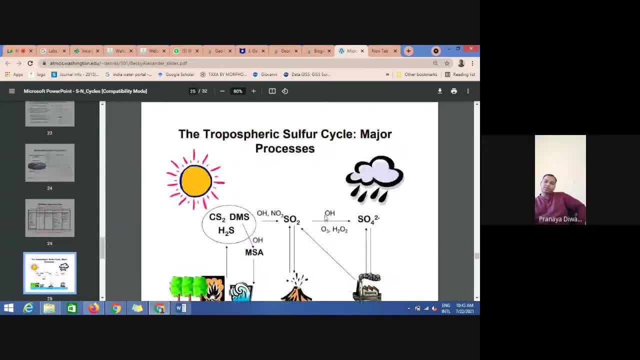 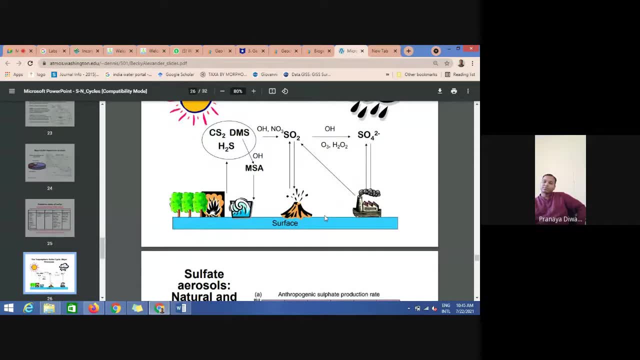 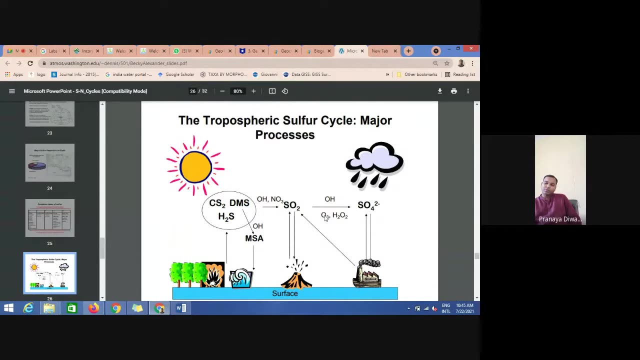 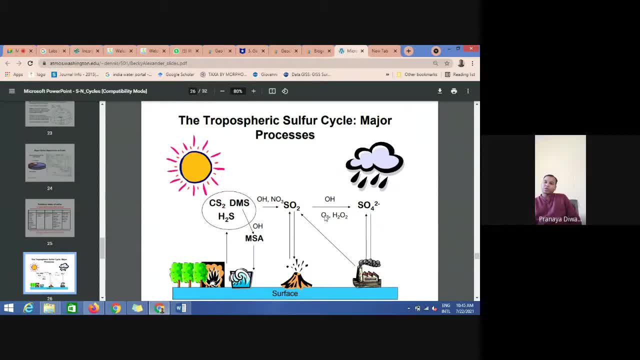 also that proper the person, that proper the person, that proper the person, so the, so the, so the can have the tropospheric sulfur, which is can have the tropospheric sulfur, which is, can have the tropospheric sulfur, which is also again, also, again, also again, going into the same process, okay, from. 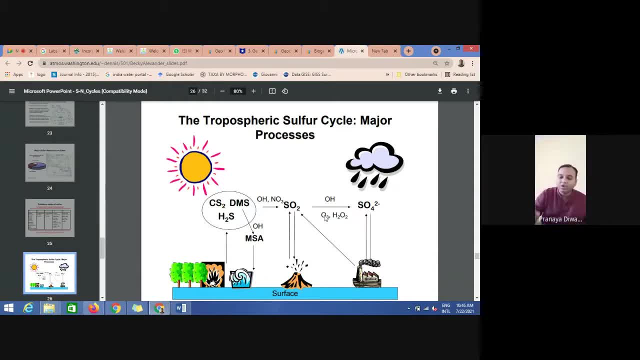 going into the same process. okay, from going into the same process. okay, from atmosphere to the atmosphere, to the atmosphere, to the lithosphere, to the biosphere, to the lithosphere, to the biosphere, to the lithosphere, to the biosphere, to the. this one so, this one, so. 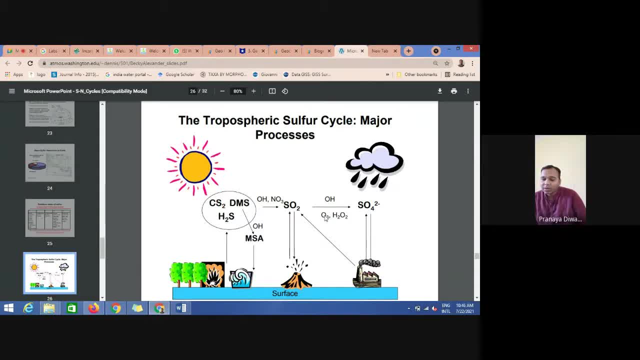 this one. so hope you know that what it means by hope you know that what it means by hope you know that what it means by biosphere, biosphere, biosphere, biosphere and atmosphere, atmosphere and this biosphere and atmosphere, atmosphere and this biosphere, and this one is common, but biosphere, uh, the 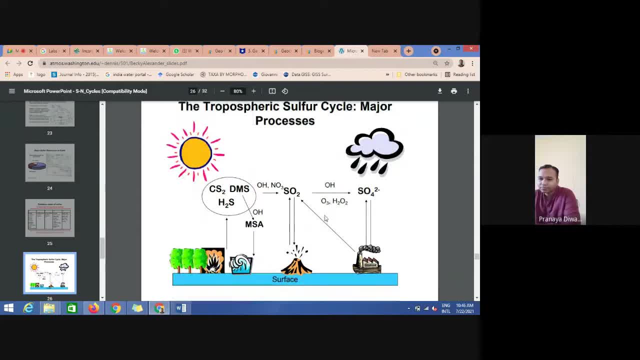 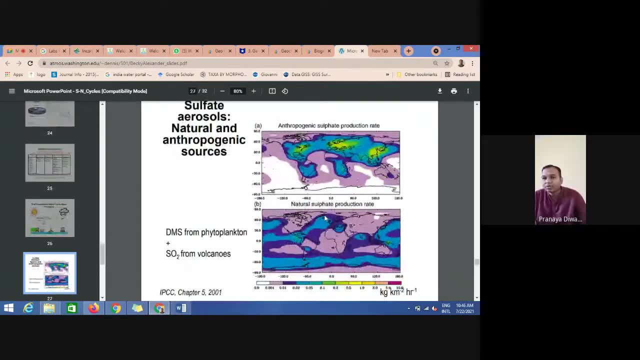 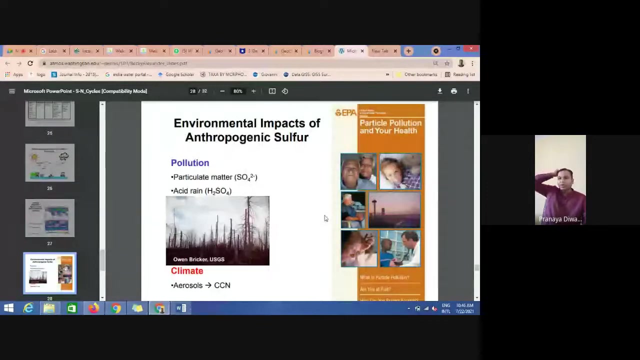 one is common, but biosphere, uh, the one is common, but biosphere, uh, the this one is also very important. then you have sulfate aerosols, then you have sulfate aerosols. then you have sulfate aerosols, natural anthropologic sources, then you have a. then you have a. 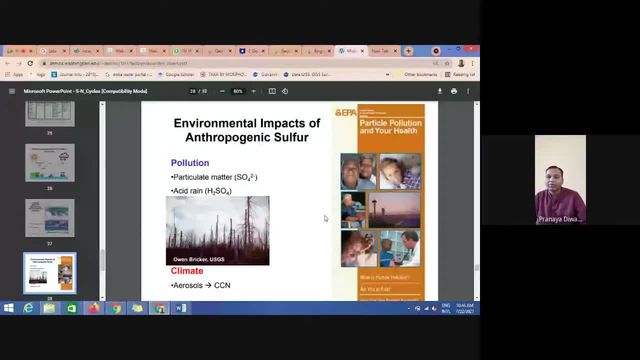 then you have a environmental, environmental, environmental, environmental environment. So, likewise, nitrogen you also have. sulphur is also having an environmental impact. What is the environmental impact of particulate matter? of particulate matter- also, you can see this one- it is a polluted, it is a polluted, so you have a pollution of sulphur when you 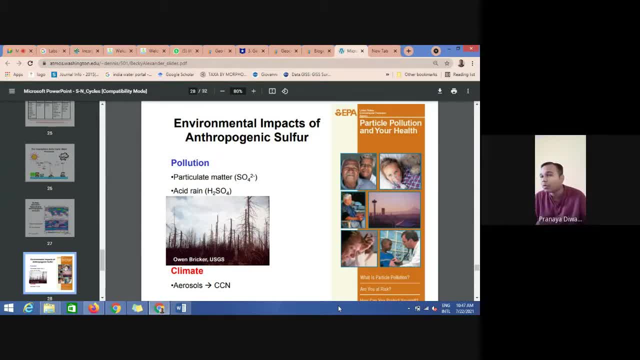 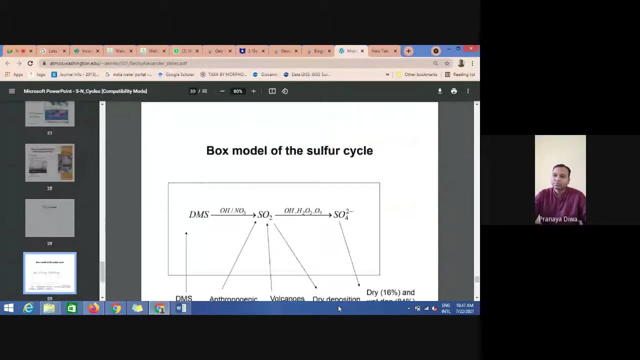 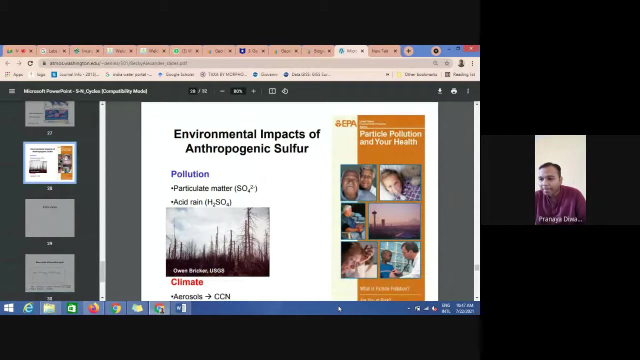 can have this billy side also, you can have a major problem of pollution. even our formula is also implemented there. but after this all, after this all, it is not going to increase. So this is, This is known as the, this is known as the cyclicity of the element. 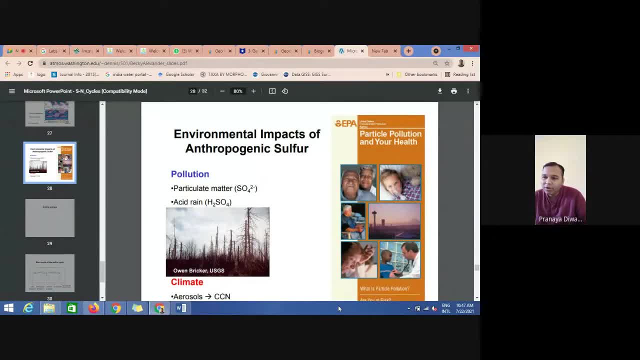 This is known as the cyclicity of the element. means from one part to another part, from another part to one part, But the component is involved and it not goes. goes out of the earth means it is remain in a system. they are reacted with the subsystem. 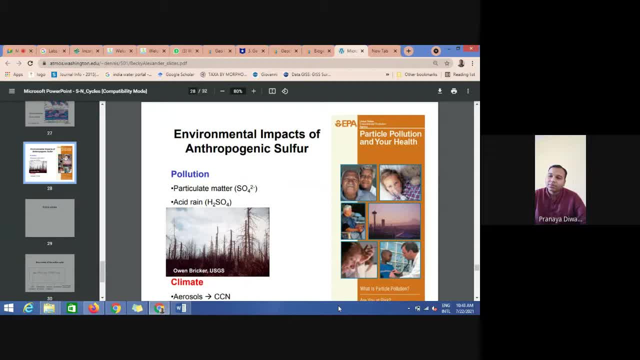 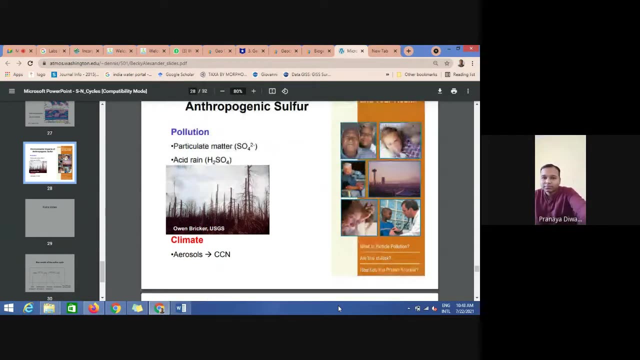 they are reacted with the subsystem and so you can have this particular matter and all. then acid rain is also common. acid rain is also common in india: 18, 1984, 83. you have one acid rain when the pollution and this all get increased. so obviously from where you? 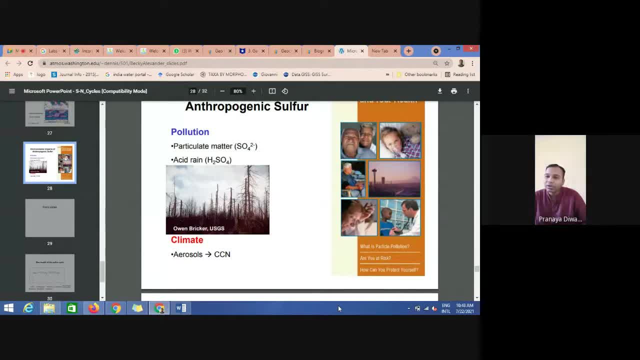 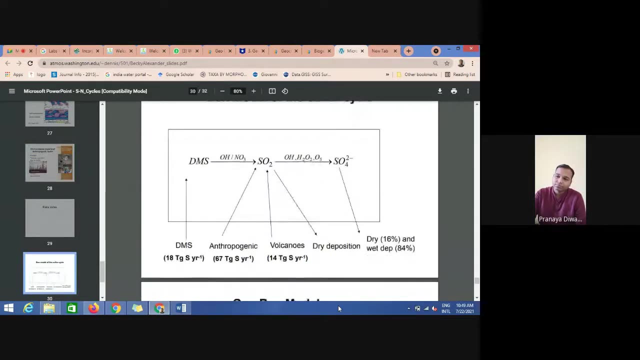 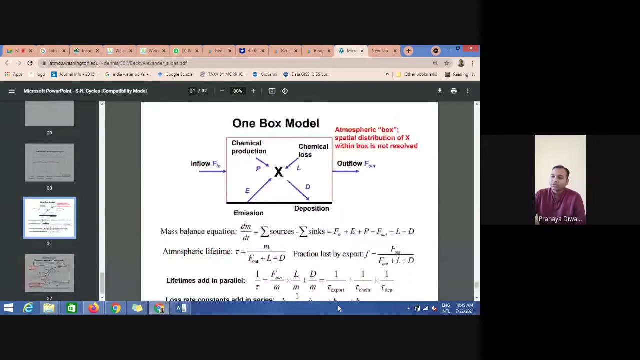 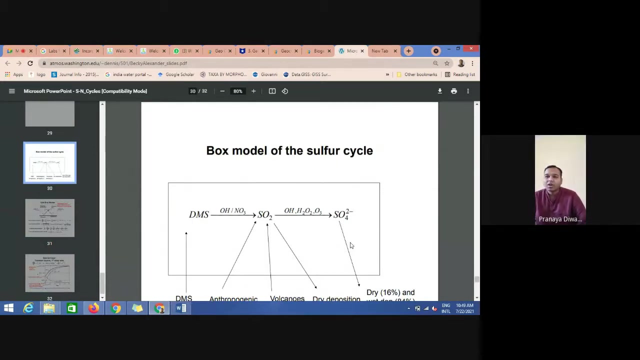 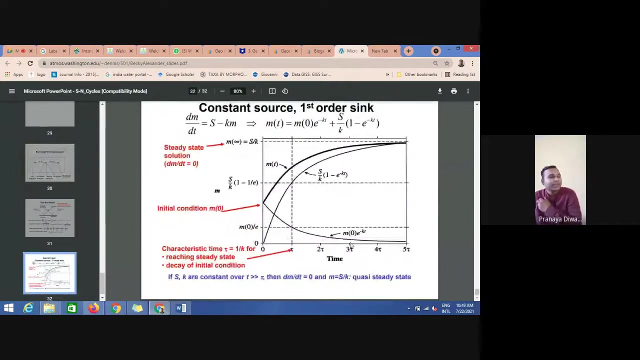 are all the clouds is making, making from the ocean river and all, if you are here, take this, not take this facility. so, so, so, so this is what this is how. and what about this lecture? about the geochemical cycling, geochemical cycling, so geochemical cycling, nothing but a cyclicity of the element. 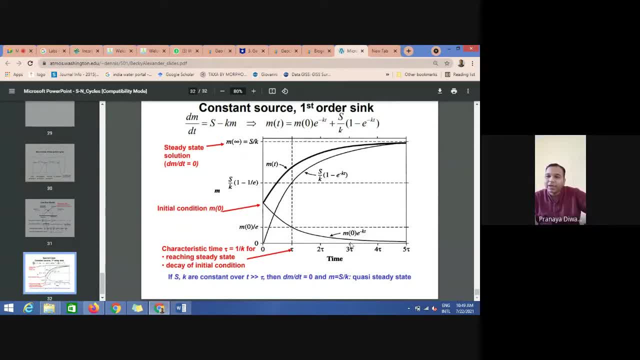 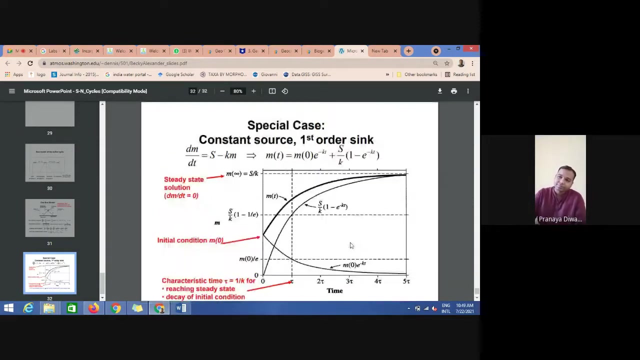 geochemical cycling, nothing but a cyclicity of the element in a particular manner that is known as the geo. so you can have initial condition m, zero, steady state solution m. so you can have the constant change and you can calculate this changes, how this changes its. so you can have the constant change and you can calculate this changes, how this changes. 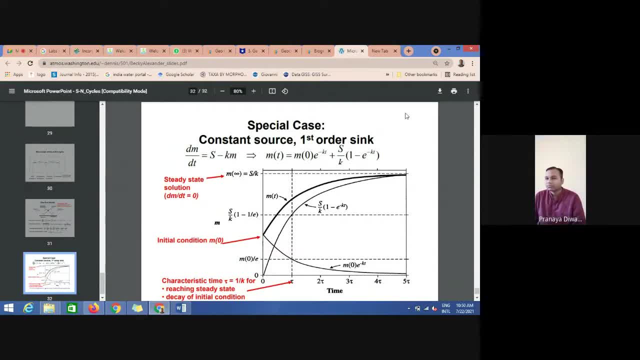 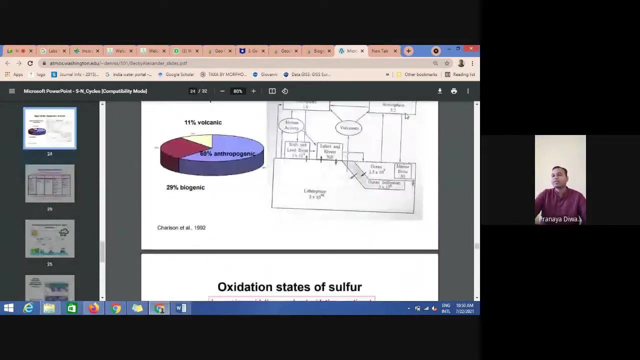 its conditions. So this is how. all about the lecture, this is all from the lecture. hope you understand and enjoy this one. have MCQ in your mind, so thank you all for listening. this one we discuss about in this lecture. we are discuss about the different kind of conditional kind. 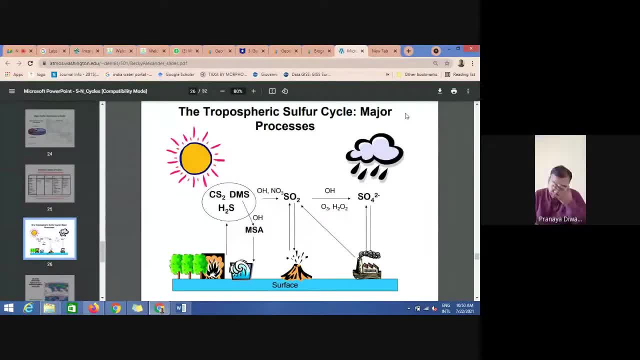 of geochemical classification, what type of element? and this one behavior of element, and this one, and tropospheric sulfur cycle, tropospheric sulfur cycle. so this all you can. you can just remember one. remember one quote that remember one quote that remember. 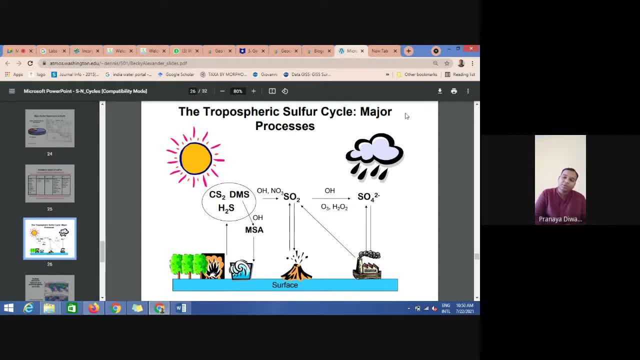 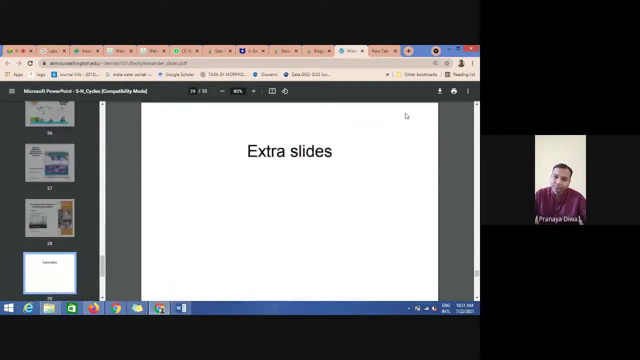 all remember one thing, one remember one thing. one remember one thing last again, again one quote, sorry, RHR. One quote, many points, reference to RHH. yes, yes, exactly, or we, that is one, baht Nair Velu Lawrence. very much, thank you very much.